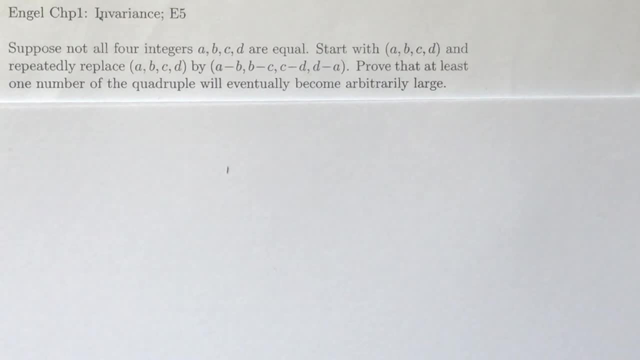 Hello fellow problem solvers. So today I'm going to be doing a problem from Engel's Problem Solving Strategies, chapter 1, on invariance, example number 5.. I suggest you try this problem out for a minimum of 10 minutes, ideally half an hour, but not more than an hour. 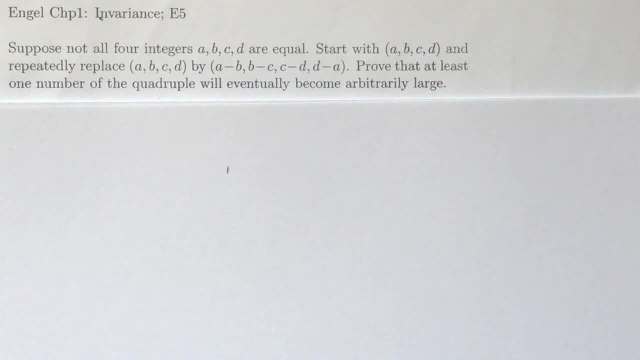 and a half. If, on the other hand, you'd like to go along with us, I suggest you take a preliminary look, put your first ideas out on paper for the next 5 to 10 minutes. So now let's begin. 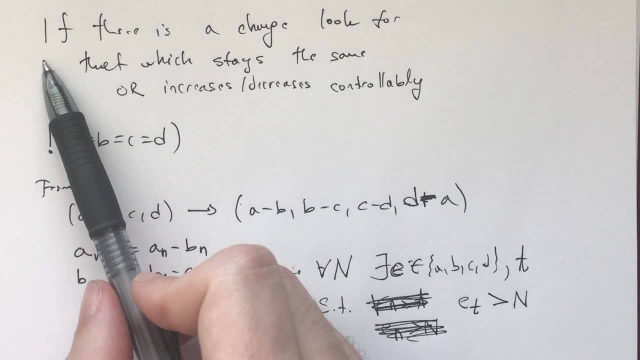 So let's repeat what invariance is the principle of invariance? If there is a change, look for things which stay the same, or this is like the extra, sort of like more advanced version of invariance is monovariance, or things that increase or decrease controllably. And now 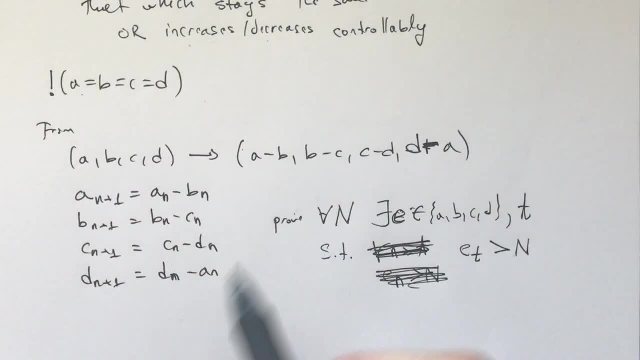 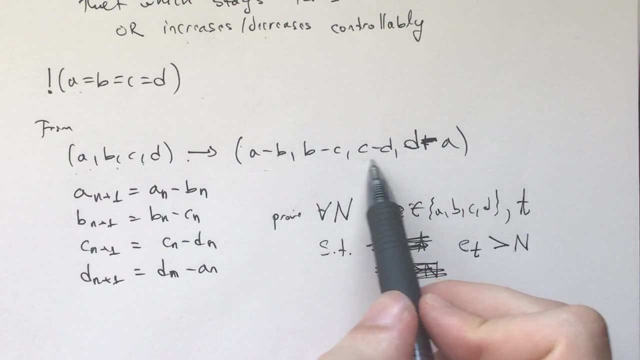 what is the problem? So we have, like all of these numbers- a, b, c, d are not all equal and at every time we get from a, b, c, d to a minus b, b minus c, c minus d and d minus a. 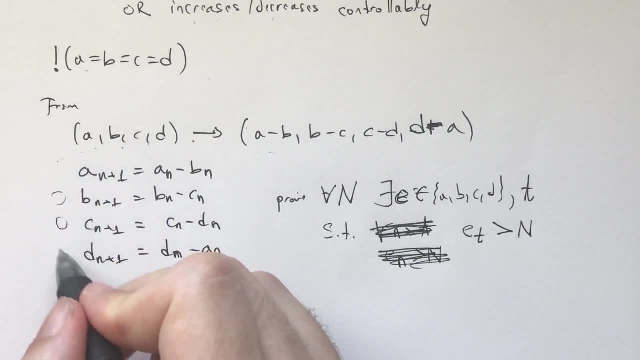 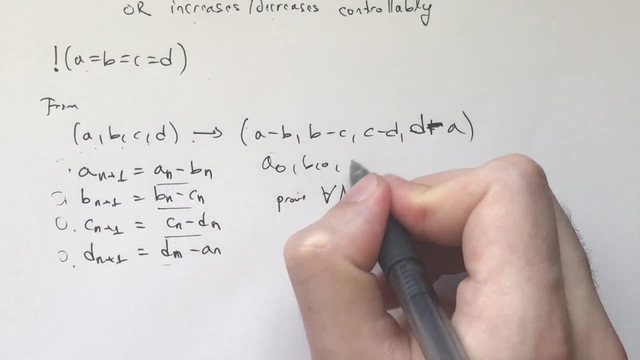 ie this sort of thing. if we call this like sequences of a and b and c and dn that satisfy this with an initial like a0,, b0,, c0, and d0- not all equal- then we must: 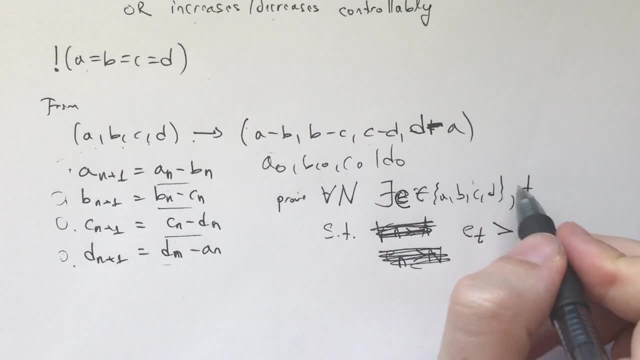 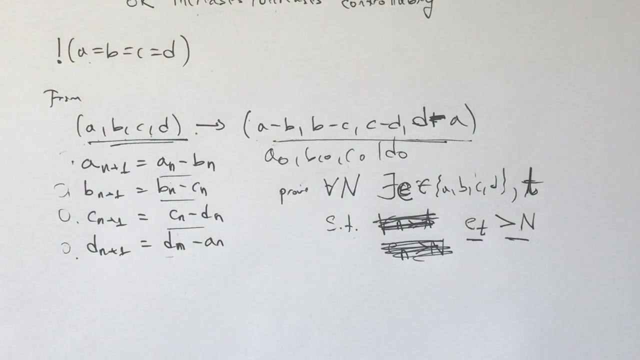 prove that for every n, there exists like an e- that's one of these- and a t, such that et is greater than n. Now, what stays the same? What changes controllably? Well, if you look at like, I invite you to take, first and foremost, take about, let's say, 5 to 10 minutes and find 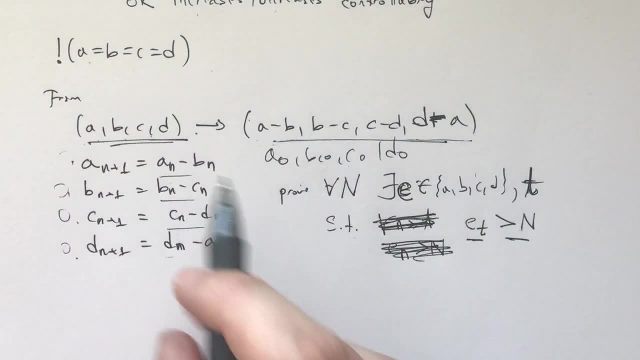 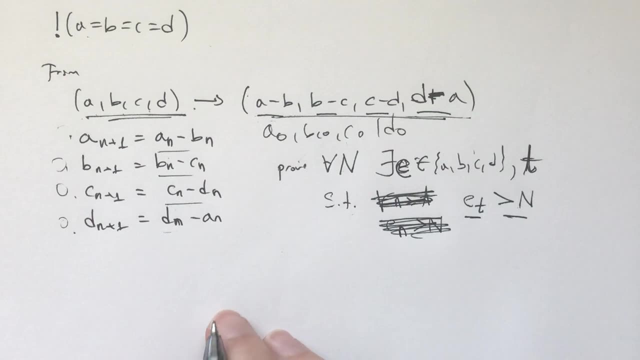 what stays the same? Anything. And what stays the same is that the sum after the initial ones, what is a minus b, b minus c, c minus d, d minus a? so the sum an plus bn plus cn. actually let's do an plus 1,. 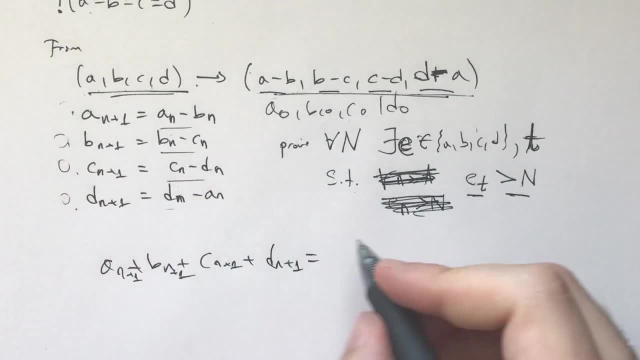 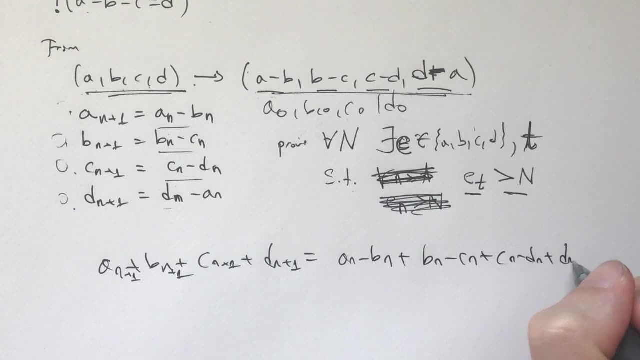 bn plus 1, cn plus 1, plus dn plus 1, is equal to what? It's equal to an minus bn plus bn minus cn, plus cn minus dn, plus dn minus an, and this is all equal to zero. So this means that 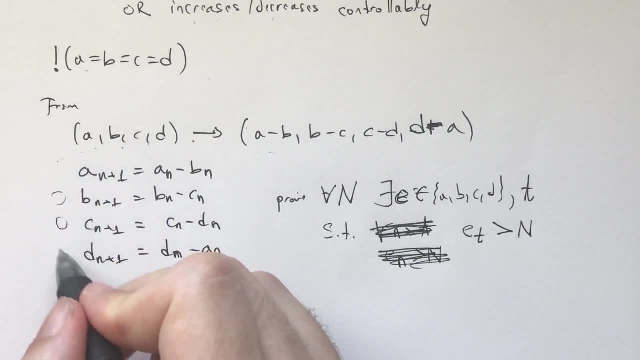 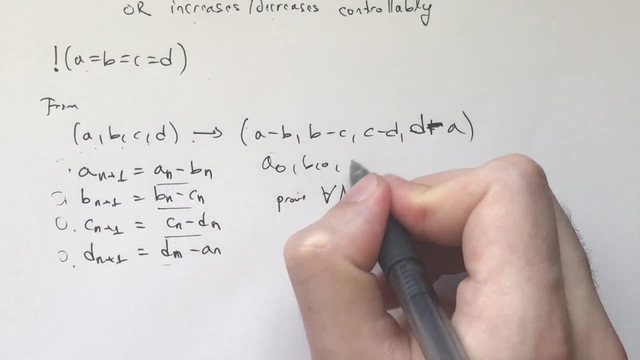 ie this sort of thing. if we call this like sequences of a and b and c and dn that satisfy this with an initial like a0,, b0,, c0, and d0- not all equal- then we must: 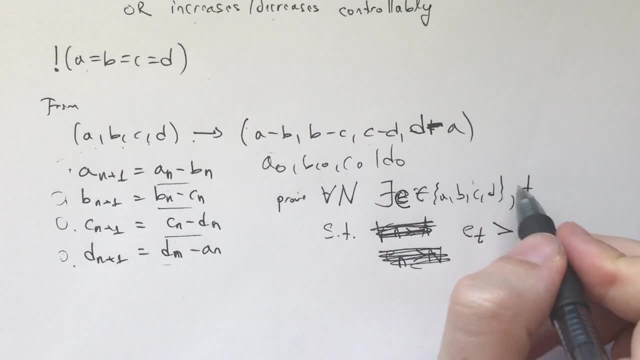 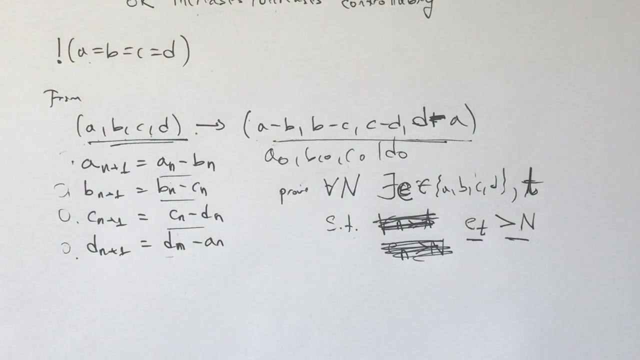 prove that for every n, there exists like an e- that's one of these- and a t, such that et is greater than n. Now, what stays the same? What changes controllably? Well, if you look at like, I invite you to take, first and foremost, take about, let's say, 5 to 10 minutes and find 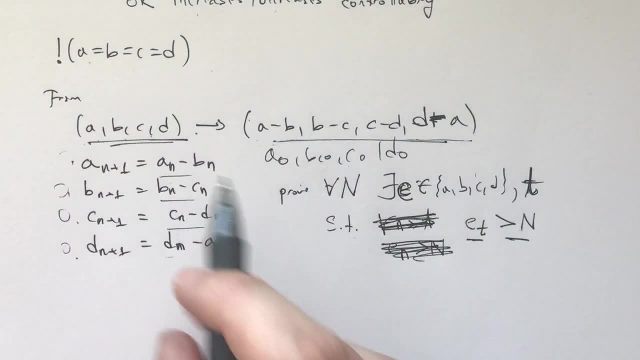 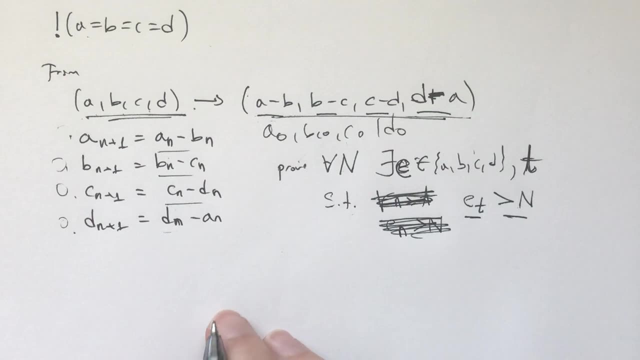 what stays the same? Anything. And what stays the same is that the sum after the initial ones, what is a minus b, b minus c, c minus d, d minus a? so the sum an plus bn plus cn. actually let's do an plus 1,. 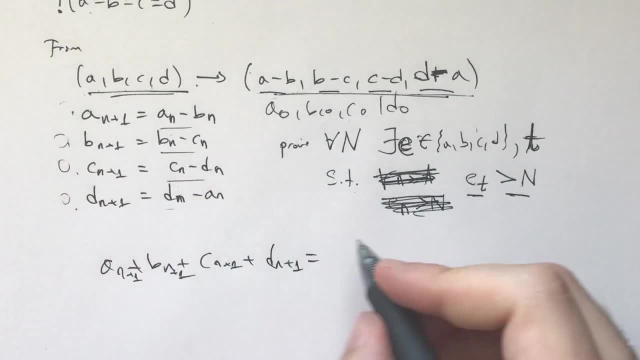 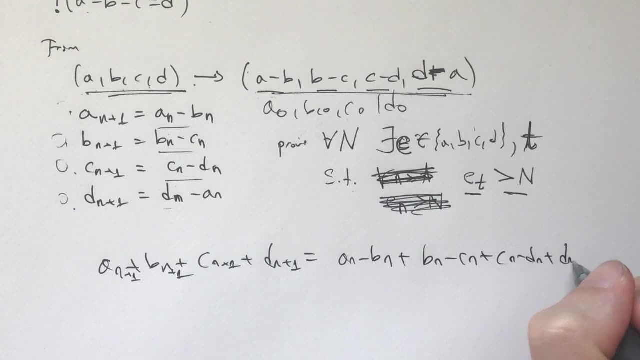 bn plus 1, cn plus 1, plus dn plus 1, is equal to what? It's equal to an minus bn plus bn minus cn, plus cn minus dn, plus dn minus an, and this is all equal to zero. So this means that 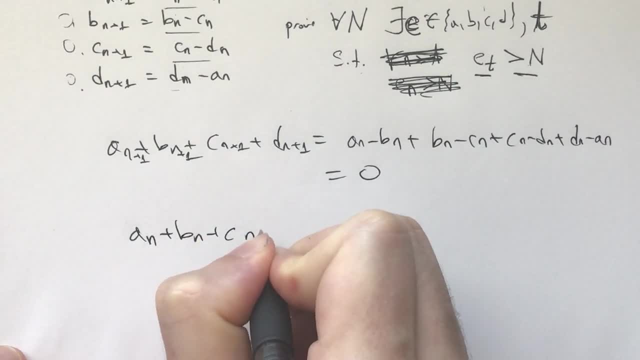 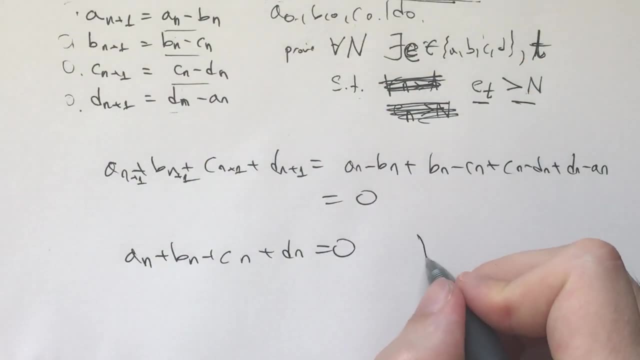 the sum an plus bn, plus cn plus dn is equal to zero, for, like, if we call the initial ones a0,, b0,, c0, d0, for all n greater than or equal to 1.. Now, how do we prove that one of them? 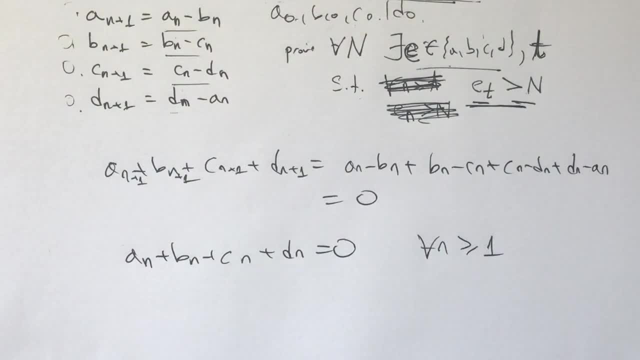 will become eventually arbitrarily large. Now I would invite you here to pause for 10 to 20 minutes and try to find a mono variant that can maybe show this to you, but also I will give you a hint. Here's the thing. 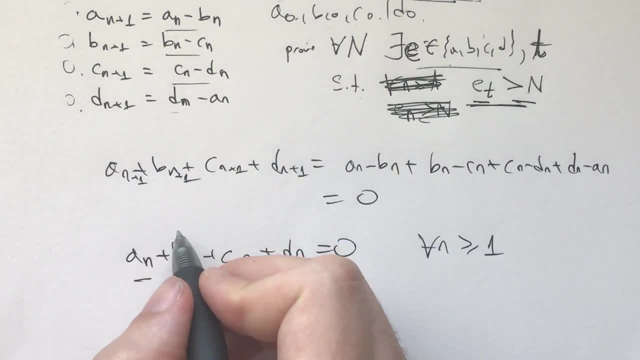 With the sum equaling zero. we don't know if each of these is like 1 minus 1, 1 minus 1,, like very small numbers, or if they are like 1,000 minus 900, minus 50 and minus 50 again. 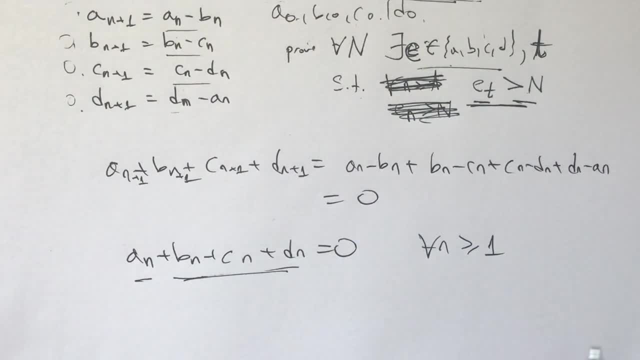 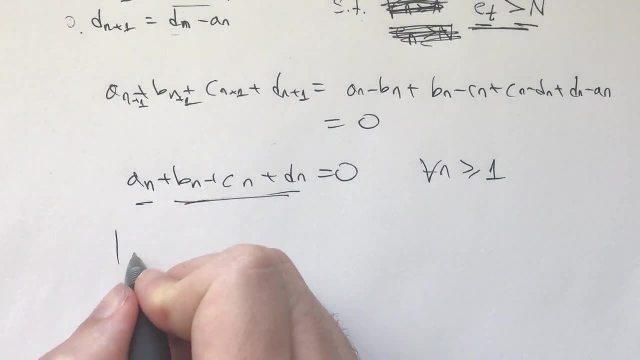 actually. So we need something that justifies, that sort of tells us how big all of these numbers are, and maybe the first sort of idea is that: absolute values. but with absolute values you have a little bit of a problem, That is, you have cases. 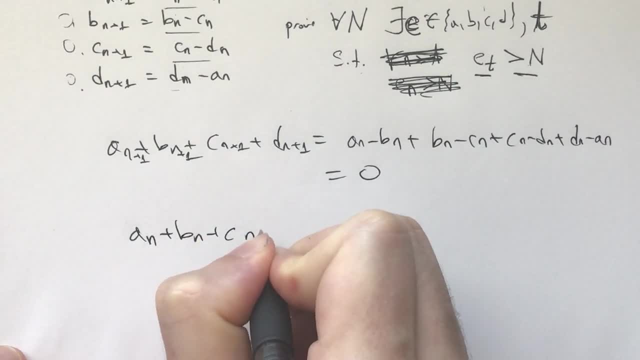 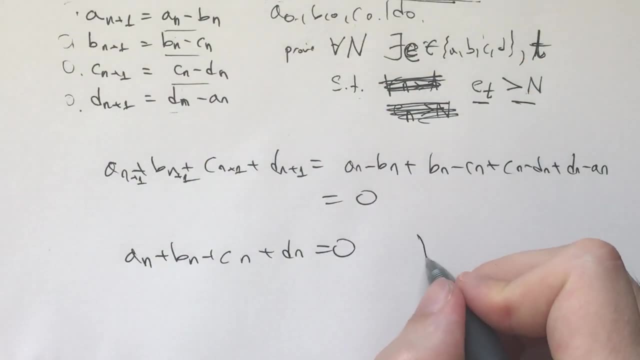 the sum an plus bn, plus cn plus dn is equal to zero, for, like, if we call the initial ones a0,, b0,, c0, d0, for all n greater than or equal to 1.. Now, how do we prove that one of them? 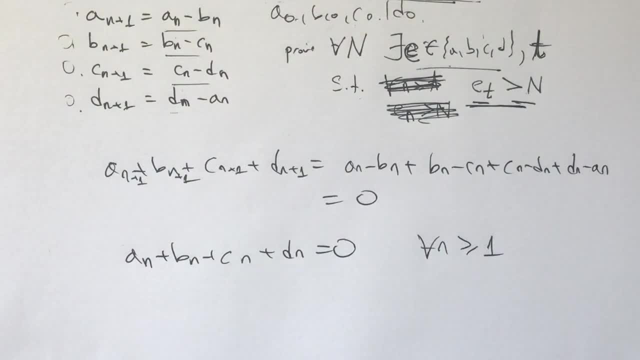 will become eventually arbitrarily large. Now I would invite you here to pause for 10 to 20 minutes and try to find a mono variant that can maybe show this to you, but also I will give you a hint. Here's the thing. 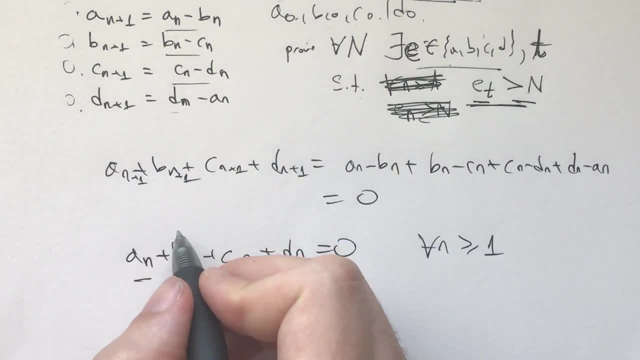 With the sum equaling zero. we don't know if each of these is like 1 minus 1, 1 minus 1,, like very small numbers, or if they are like 1,000 minus 900, minus 50 and minus 50 again. 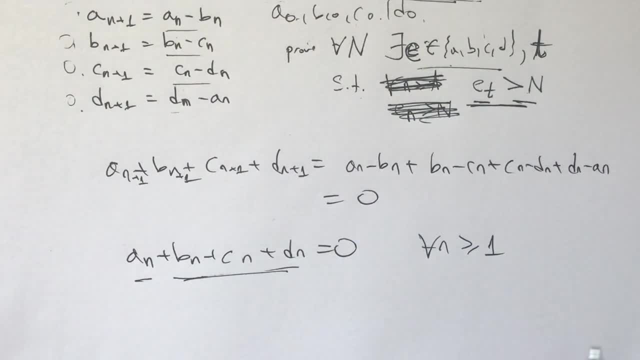 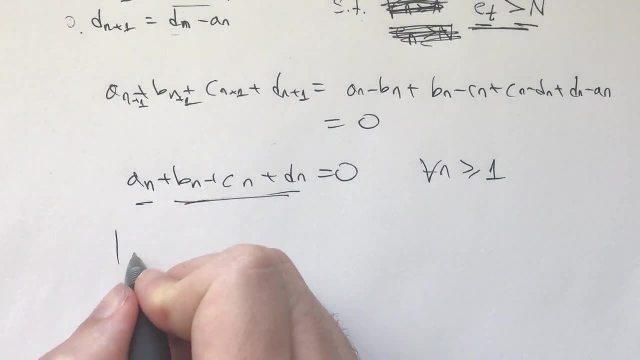 actually. So we need something that justifies, that sort of tells us how big all of these numbers are, and maybe the first sort of idea is that: absolute values. but with absolute values you have a little bit of a problem, That is, you have cases. 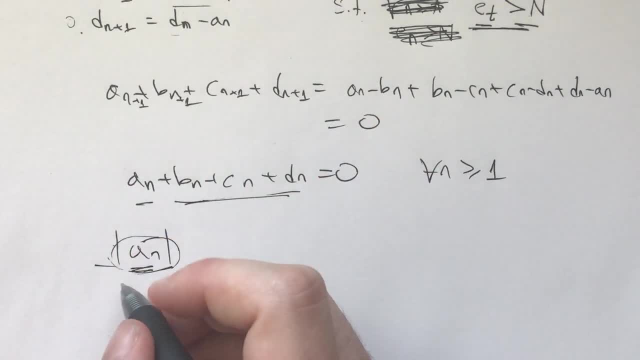 That may or may not be difficult to work with, but is there a different way than looking at the absolute value of all of these numbers? Is there something else? you can look at another type of sum, And here I invite you to pause for 5 to 10 minutes and try to find another. 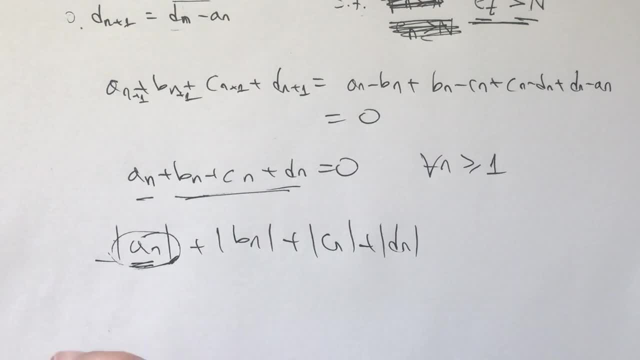 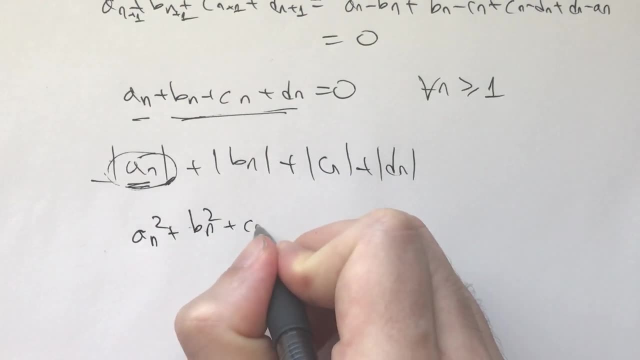 sort of mono variant, and here's that idea. So instead of absolute values to look at size, we can look at the squares, the sum of these numbers as squares, and we need to show that this sort of sum of squares is not a monovariant. So instead of absolute values, we can look at: 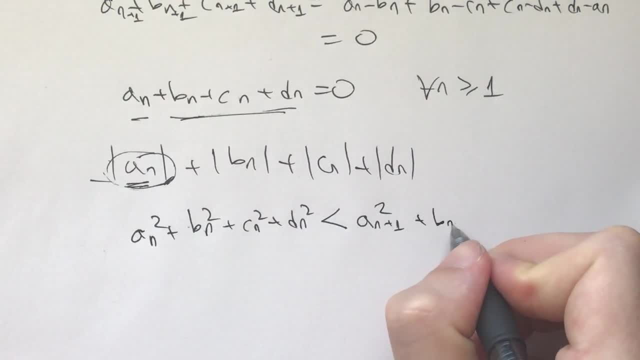 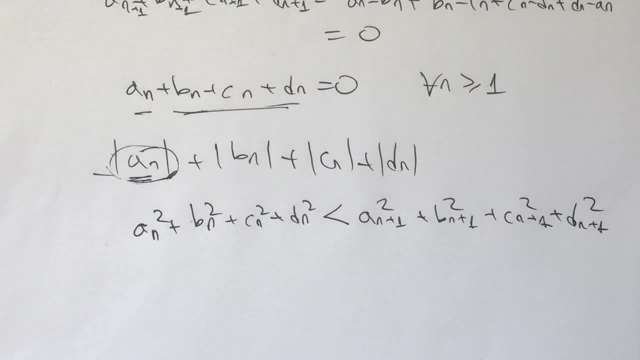 squares. If we show that it always increases, then what we are showing is that because it's always increasing, then at least one of these numbers must be arbitrarily large, and we can show that, and I invite you to pause for 5 minutes and try to prove this. and here's the proof. 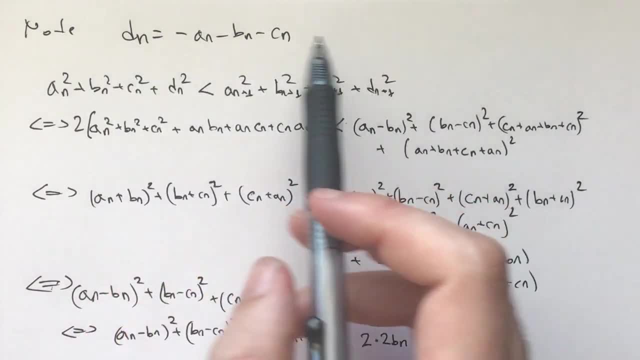 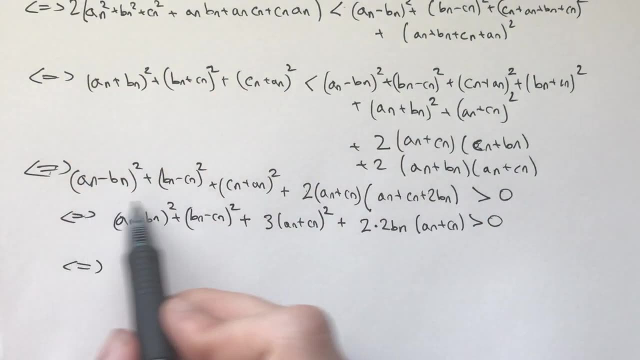 So this is the algebraic manipulation: right dn is negative, an negative bn, negative cn. and then what you get from here? you get this, you get this is all true, if and only if. These are all if and only if statements. if and only if this is true. 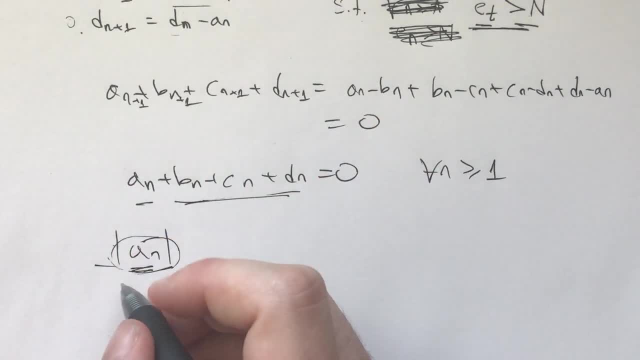 That may or may not be difficult to work with, but is there a different way than looking at the absolute value of all of these numbers? Is there something else? you can look at another type of sum, And here I invite you to pause for 5 to 10 minutes and try to find another. 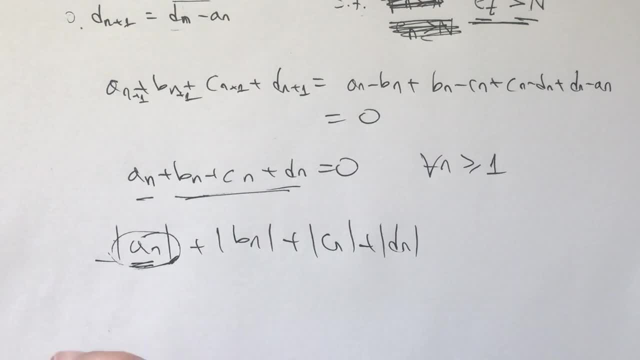 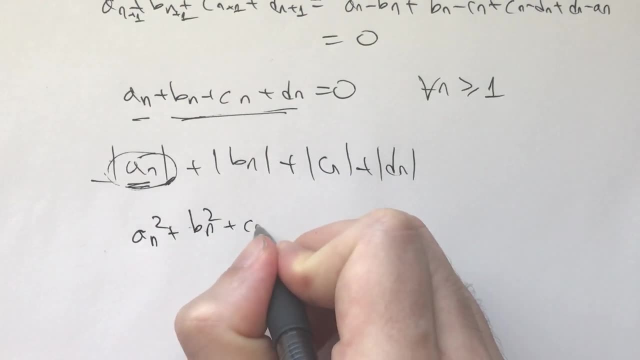 sort of mono variant, and here's that idea. So instead of absolute values to look at size, we can look at the squares, the sum of these numbers as squares, and we need to show that this sort of sum of squares is not a monovariant. So instead of absolute values, we can look at: 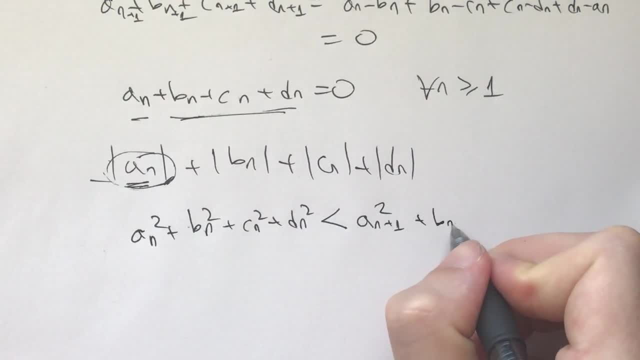 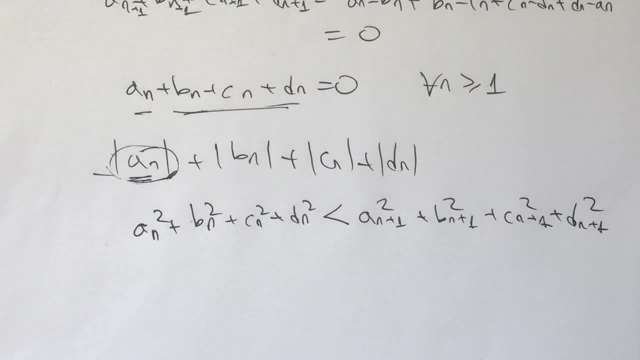 squares. If we show that it always increases, then what we are showing is that because it's always increasing, then at least one of these numbers must be arbitrarily large, and we can show that, and I invite you to pause for 5 minutes and try to prove this. and here's the proof. 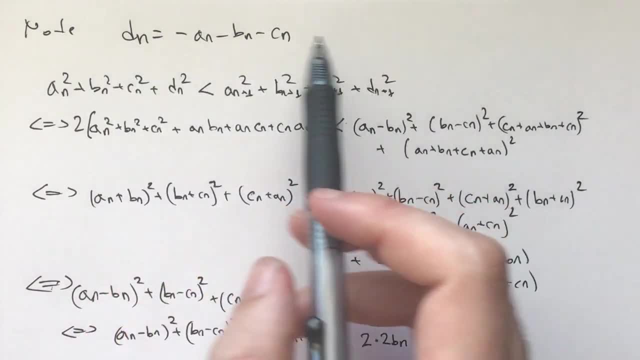 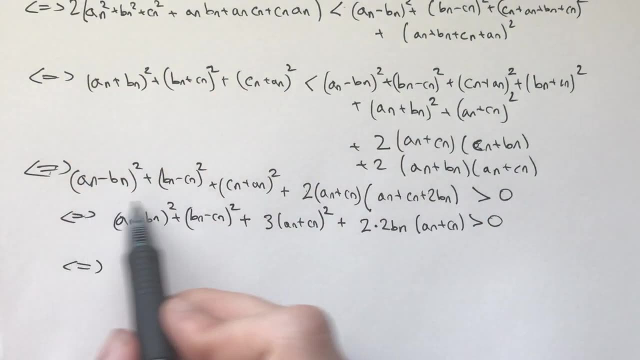 So this is the algebraic manipulation: right dn is negative, an negative bn, negative cn. and then what you get from here? you get this, you get this is all true, if and only if. These are all if and only if statements. if and only if this is true. 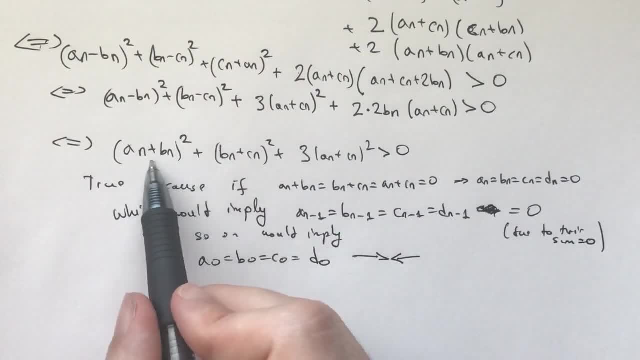 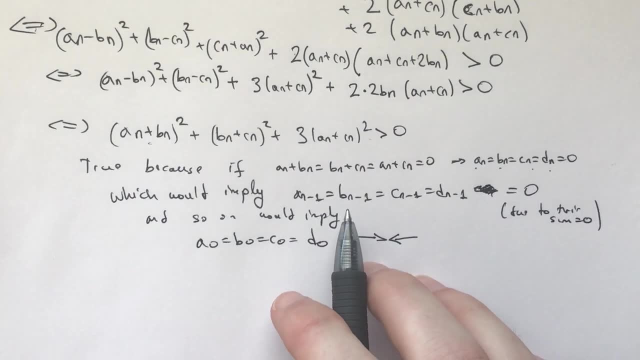 With the final thing being true, if, and only if, which implies this, which is true because if all of these were zero, that would imply a and b and c and dn were all equal to zero, which would imply that the previous ones were equal, and then equal to zero due to their sum being zero, which would 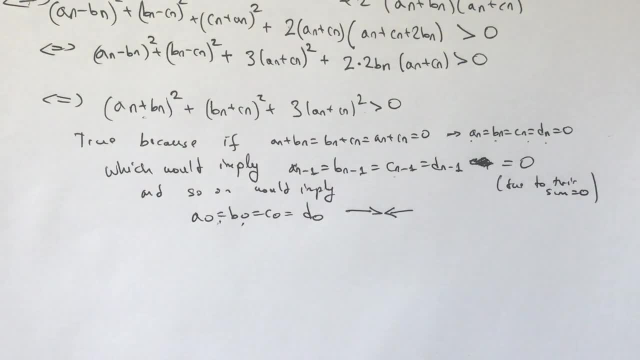 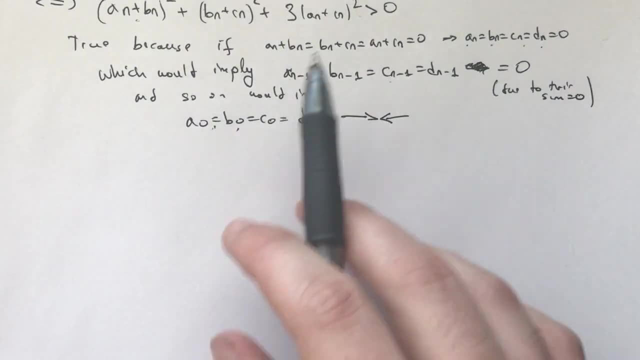 finally imply, just going backwards, a zero is equal to b zero is equal to c zero is equal to d zero, which is a contradiction by the problem statement. And now, with this, I invite you to take 5-10 minutes and formally prove that one of these numbers will eventually become true. 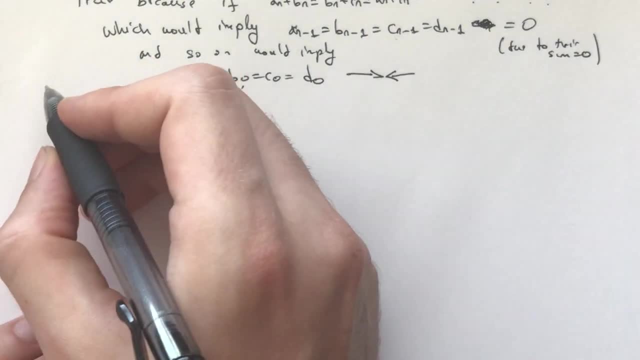 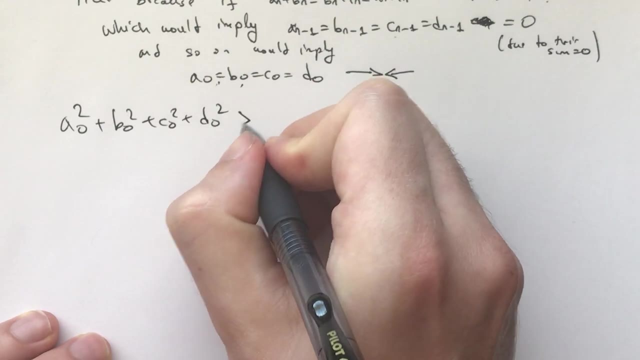 arbitrarily large. So here's the next step. Namely now you know that we know that a- zero squared- plus b- zero squared, plus c- zero squared. plus d- zero squared is greater than or equal to one, but let's just make it strictly greater than zero. And so we also know that an plus one. 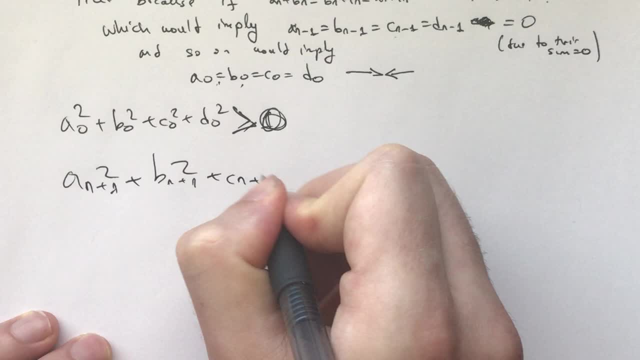 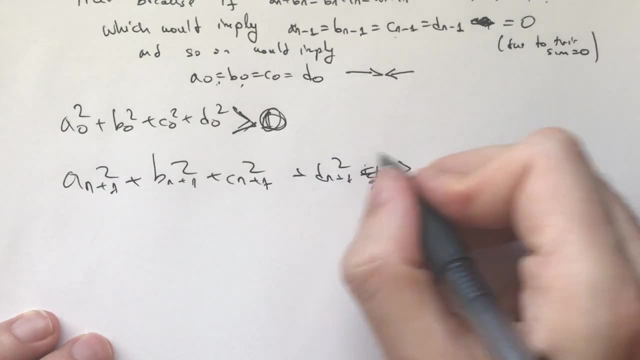 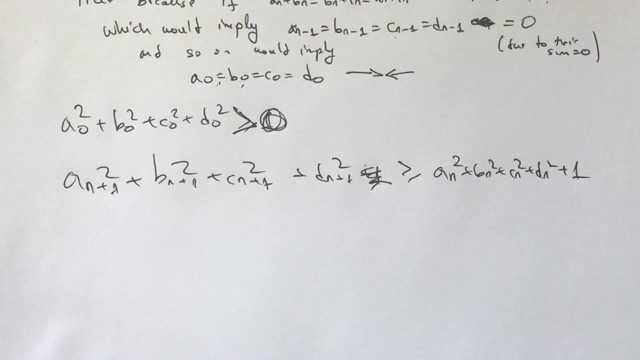 squared plus bn plus one, squared plus cn plus one. squared plus dn plus one squared plus one, is greater than or equal to a. actually, no, this minus one. actually an squared plus bn. squared plus cn. squared plus dn squared plus one, because we're in the natural number, actually not natural. 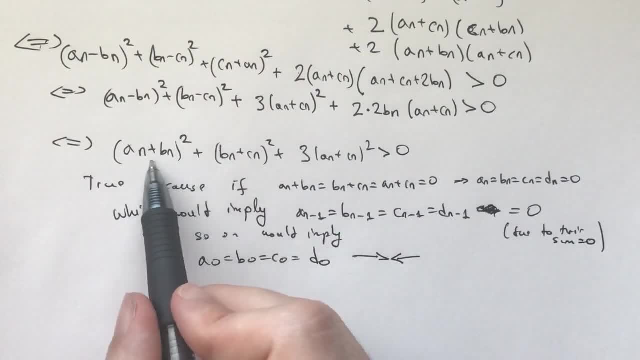 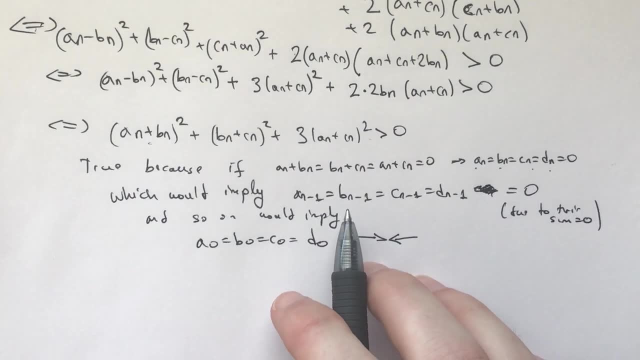 With the final thing being true, if, and only if, which implies this, which is true because if all of these were zero, that would imply a and b and c and dn were all equal to zero, which would imply that the previous ones were equal, and then equal to zero due to their sum being zero, which would 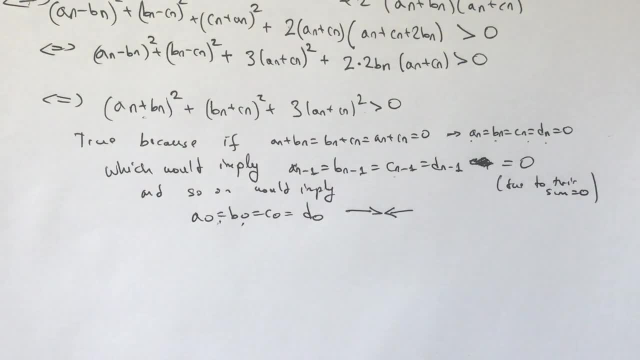 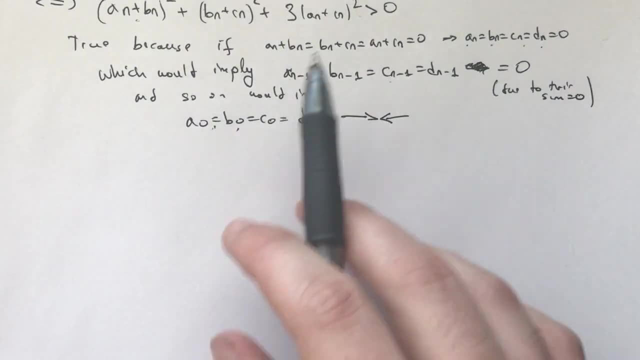 finally imply, just going backwards, a zero is equal to b zero is equal to c zero is equal to d zero, which is a contradiction by the problem statement. And now, with this, I invite you to take 5-10 minutes and formally prove that one of these numbers will eventually become true. 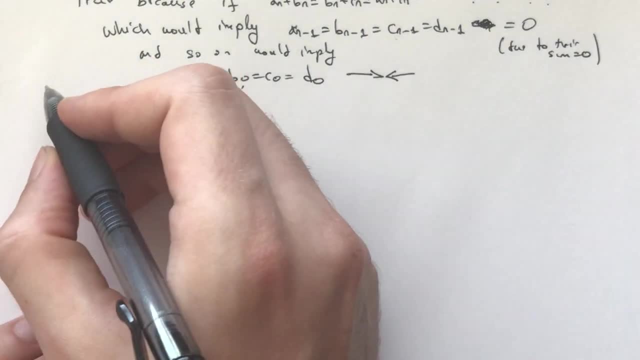 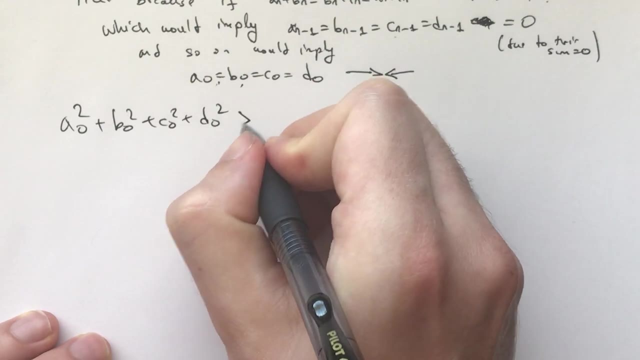 arbitrarily large. So here's the next step. Namely now you know that we know that a- zero squared- plus b- zero squared, plus c- zero squared. plus d- zero squared is greater than or equal to one, but let's just make it strictly greater than zero. And so we also know that an plus one. 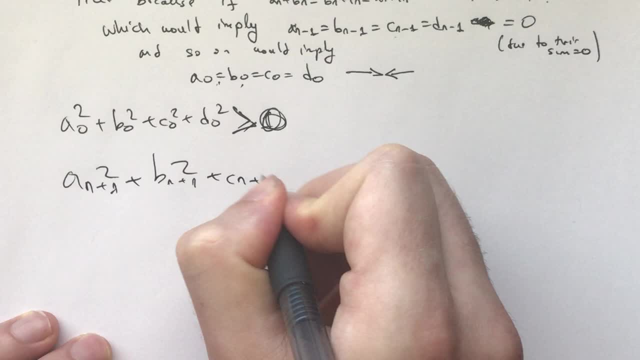 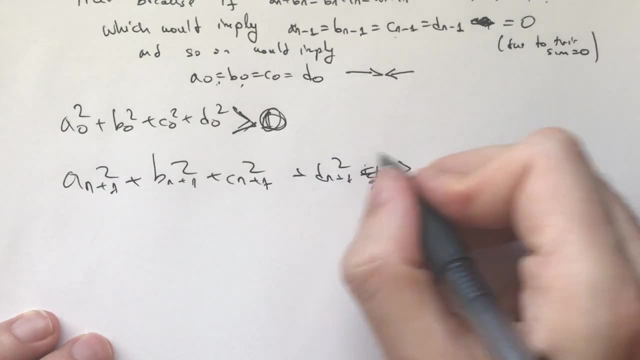 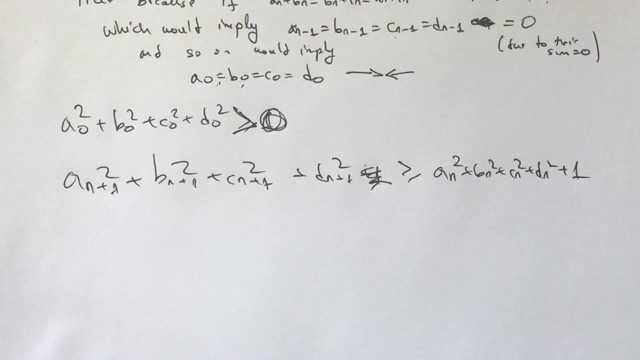 squared plus bn plus one, squared plus cn plus one. squared plus dn plus one squared plus one, is greater than or equal to a. actually, no, this minus one. actually an squared plus bn. squared plus cn. squared plus dn squared plus one, because we're in the natural number, actually not natural. 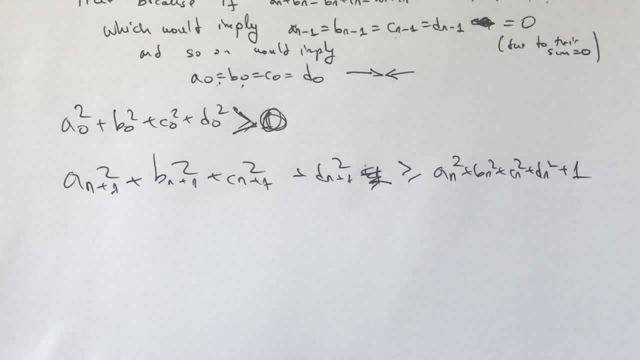 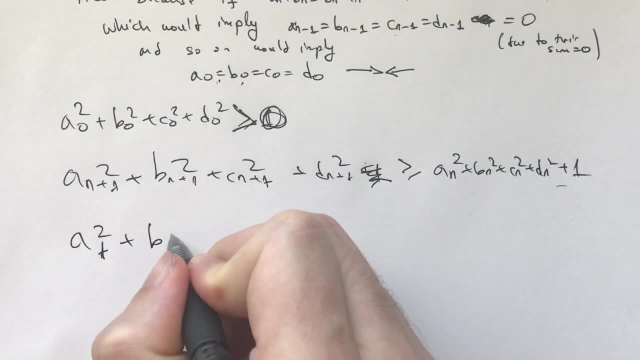 numbers, but the positive integers because of these squares. but we're in the integers, so we can add a one here. And with these two things we know that at squared plus bt, squared plus ct, squared plus dt, squared is going to be strictly greater than t. And now with this let's take 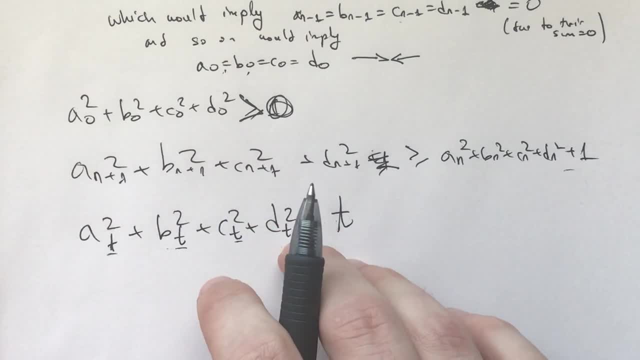 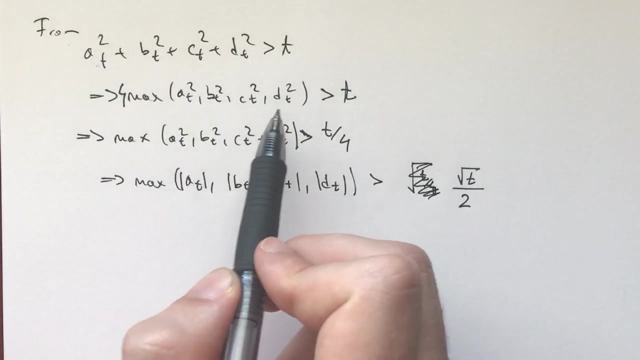 a specific t. And if you haven't come this far, I actually invite you to take another three to five minutes and be careful and try to prove the claim of the problem. Here's the next step. So, from the sum of squares greater than t, we have that four times the biggest one of these. 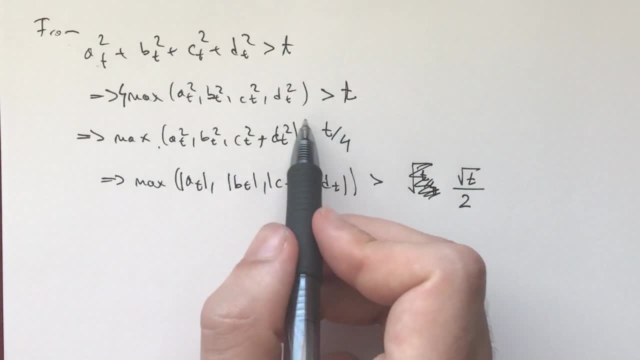 squares is greater than t, which means that the biggest one is greater than t over four, which means that the absolute value of the biggest one is greater than the square root of t over two. Now, if the absolute value of the max is equal to that number, 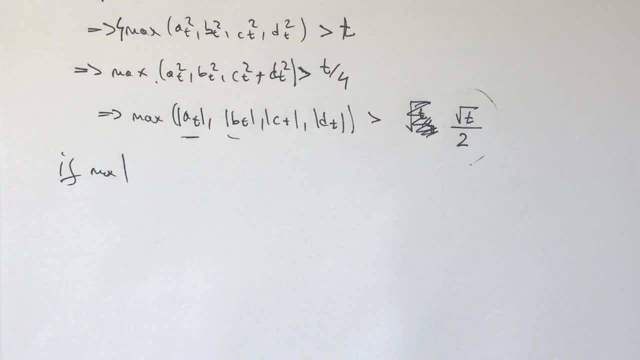 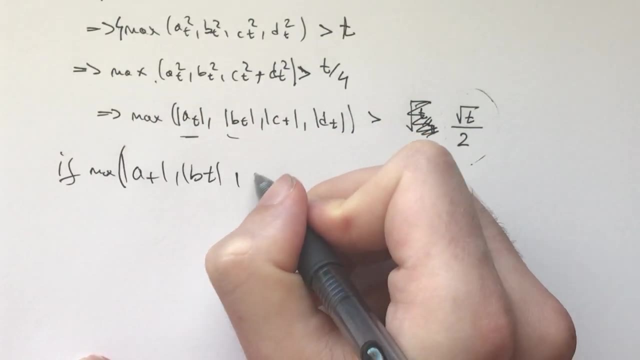 ie if the number is positive, we are done. If it's negative, we have another case that we need to take care of And how we do that. we say if max of at bt, ct and dt if this is equal to. 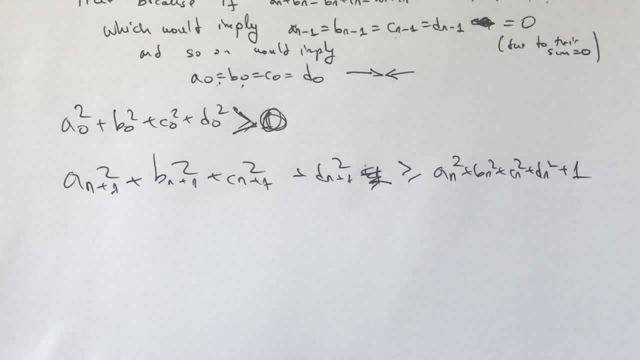 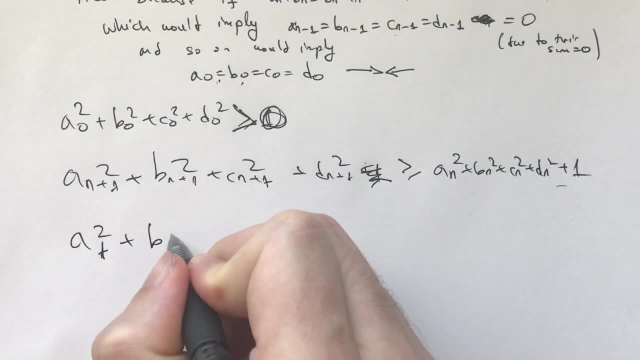 numbers, but the positive integers because of these squares. but we're in the integers, so we can add a one here. And with these two things we know that at squared plus bt, squared plus ct, squared plus dt, squared is going to be strictly greater than t. And now with this let's take 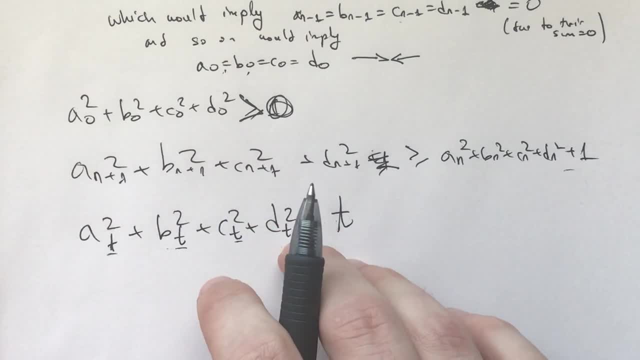 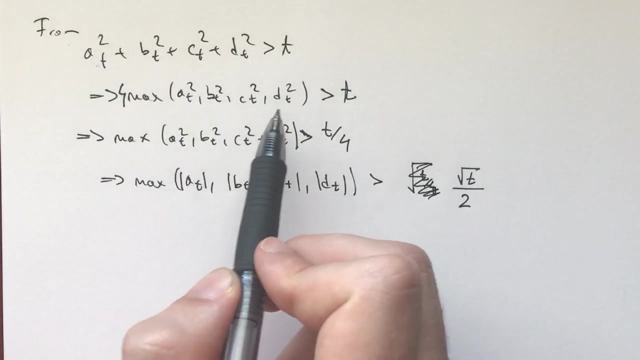 a specific t. And if you haven't come this far, I actually invite you to take another three to five minutes and be careful and try to prove the claim of the problem. Here's the next step. So, from the sum of squares greater than t, we have that four times the biggest one of these. 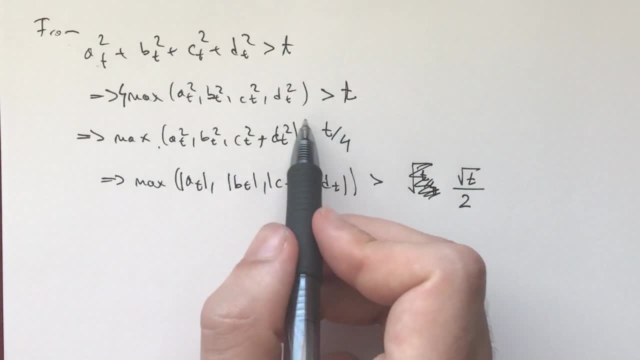 squares is greater than t, which means that the biggest one is greater than t over four, which means that the absolute value of the biggest one is greater than the square root of t over two. Now, if the absolute value of the max is equal to that number, 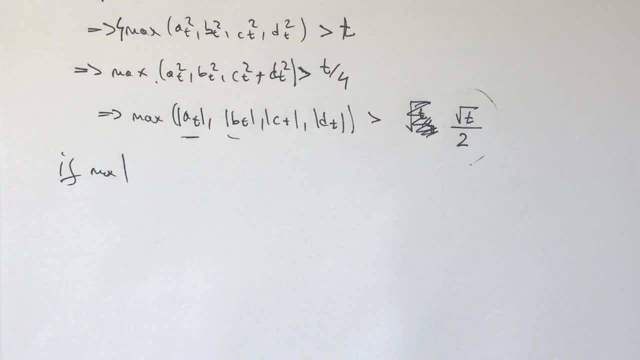 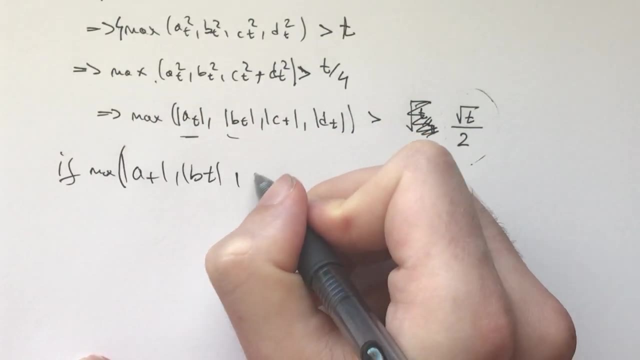 ie if the number is positive, we are done. If it's negative, we have another case that we need to take care of And how we do that. we say if max of at bt, ct and dt if this is equal to. 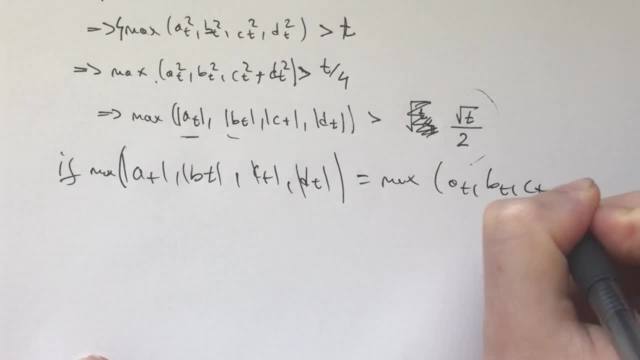 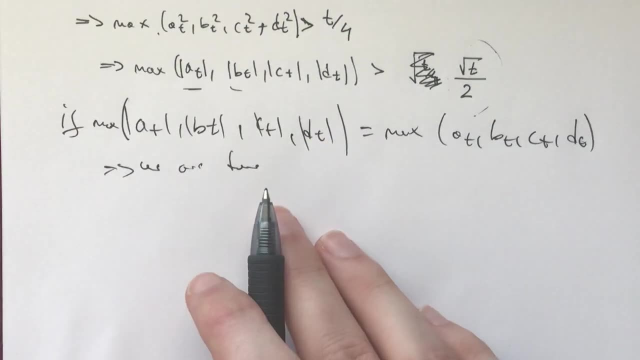 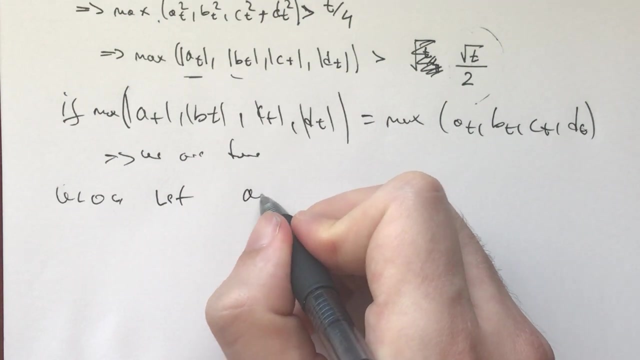 the max of at bt, ct and dt. that implies then we are done. However, if, on the other hand, the max of this isn't the one of the max, then let's assume, without loss of generality, let the negative, let at, be less than zero and the max of all of these numbers be equal. 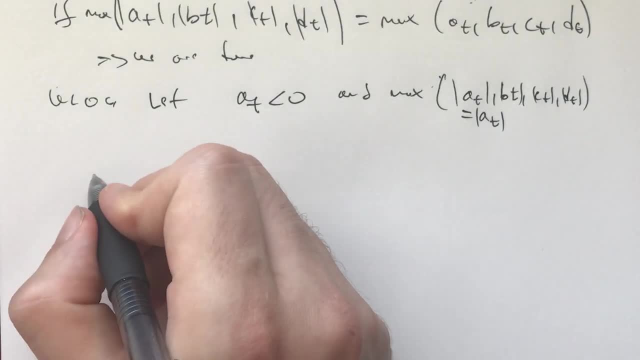 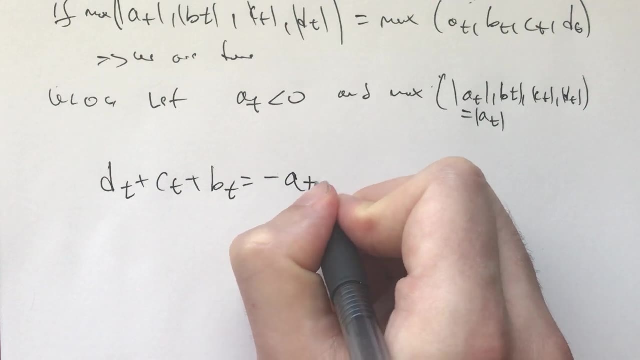 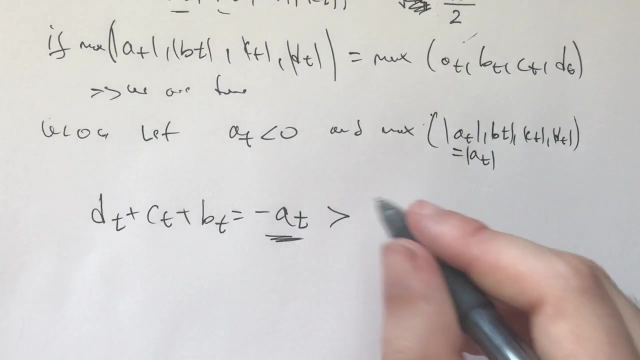 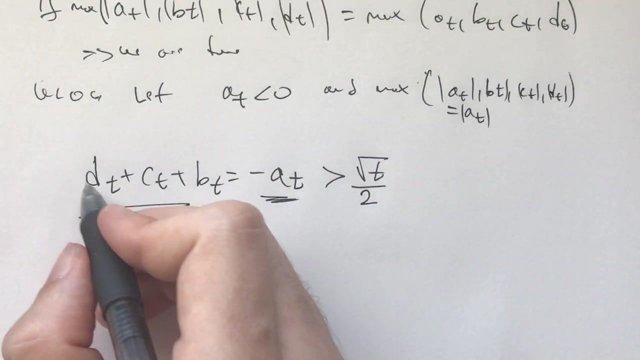 to at. Then what we have is, from dt plus ct plus bt is equal to negative at which, now we know, because this negative is the absolute value, we know this negative thing is greater than the square root of t over two. And now we know that the biggest one of these is what? Well, we know that three times that.